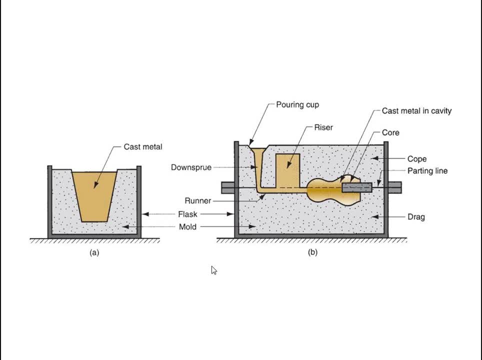 So, in order to make some casting at first, the metal that can be iron, aluminium, steel or other metals- that is at first made liquid by heating, by adding temperature or by adding heat. Then, when it becomes liquid, it is poured in mold. So it is poured in this way, in this mold, or in this mold. 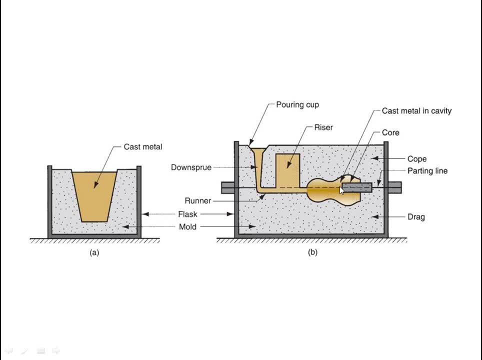 So when it is poured, it follows this way and goes here and the extra liquid Or extra casted materials are stored here, Are stored here. So when the casted material or the liquid becomes solid, it shrinks And in order to fill up this gap, for the shrinkage, there may become some gap and in order to fill up those gaps, some metals come from the riser and fill up those gaps. 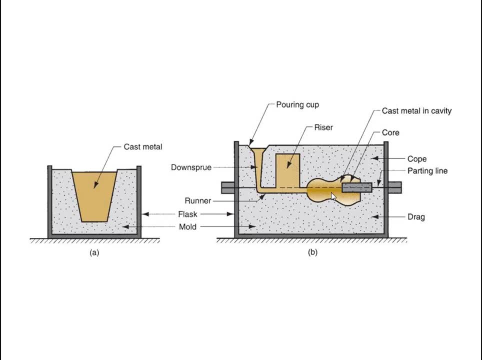 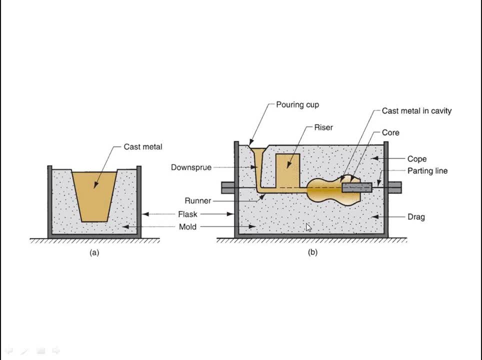 So in that case the mold can be two types. One is permanent mold and another one is temporary mold or one time mold. So the temporary mold is basically made of sand or plaster And is normally used for one time molding. For this kind of casting it is usually the temporary mold and after making this type of product the mold is destroyed or sacrificed. 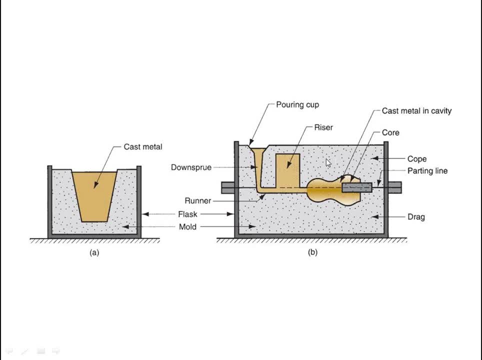 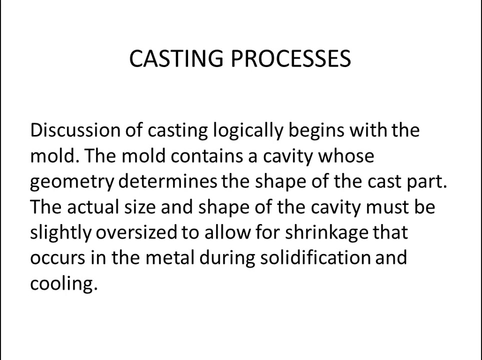 And for permanent mold there are two parts. The first one is called pope and the lower portion is called rug And they are joined by some adhesives And after making any kind of product the cope and rug is isolated. So if we go for literally, casting process, Discussion of casting- 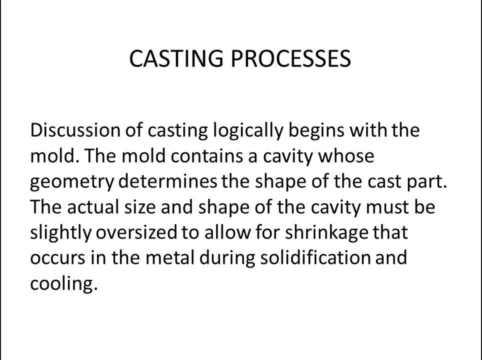 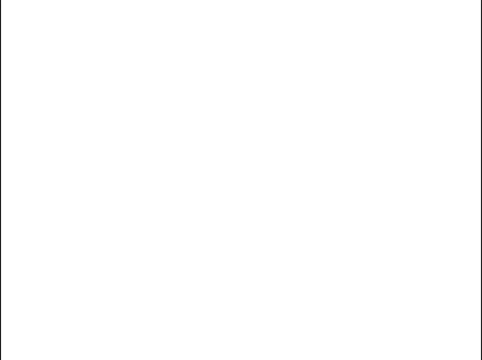 logically begins with the mold. The mold contains a cavity whose geometry determines the shape of the cast part. The actual size and shape of the cavity must be slightly oversized to allow for shrinkage that occurs in the metal during solidification and cooling. So this shape should 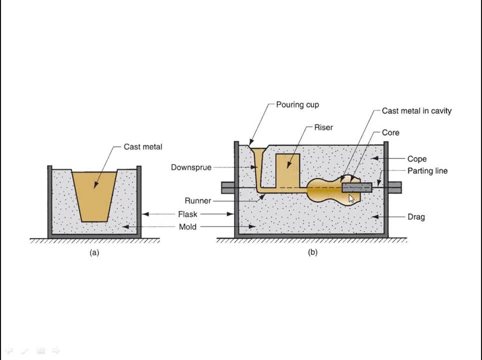 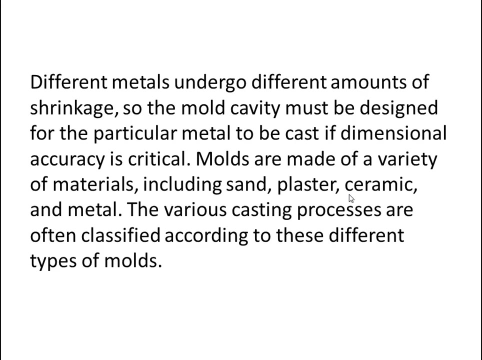 be more than the actual size of the casted product. and after we get the product we should do some machining processes, and that can be cleaning or other processes. Different metals undergo different amounts of shrinkage, So the mold cavity must be slightly oversized to allow for. 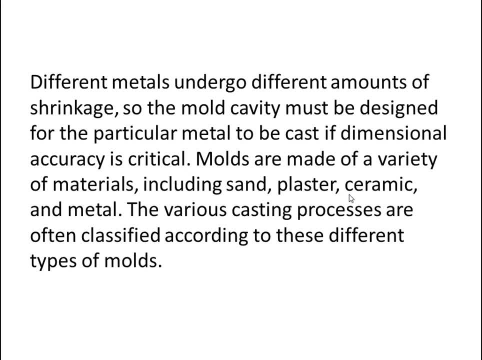 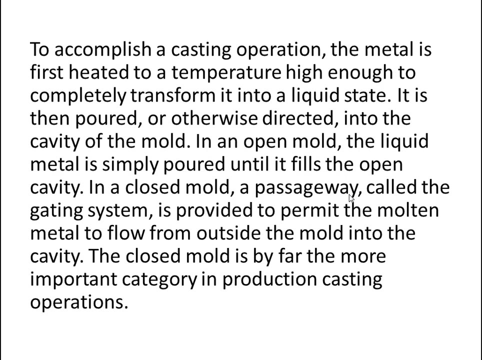 be designed for the particular metal to be cast. if dimensional accuracy is critical, Molds are made of a variety of materials, including sand, plaster, ceramic and metal. The various casting processes are often classified according to these different types of molds. To accomplish a casting operation, the metal is first heated to a temperature high enough. 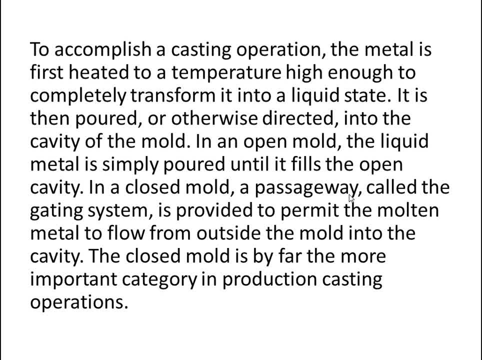 to completely transform it into a liquid state. It is then poured or otherwise directed into the cavity of the mold. In an open mold, the liquid metal is simply poured until it fills the open cavity. In a closed mold, a passageway called the gating system is provided to permit the molten. 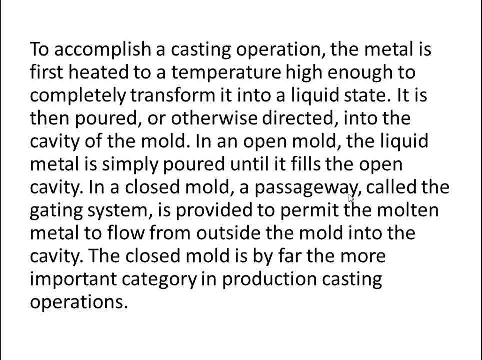 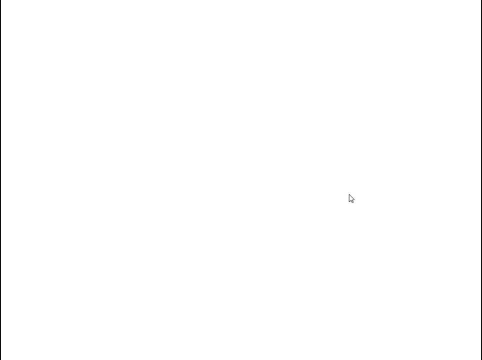 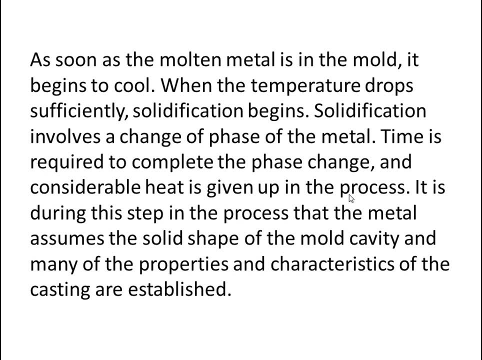 metal to flow from outside the mold into the cavity. The closed mold is by far more important category in the production category. As soon as the molten metal in the mold is begins to cool, the temperature drops sufficiently, Solidification begins. Solidification involves a change of phase of the metal. Time is required. 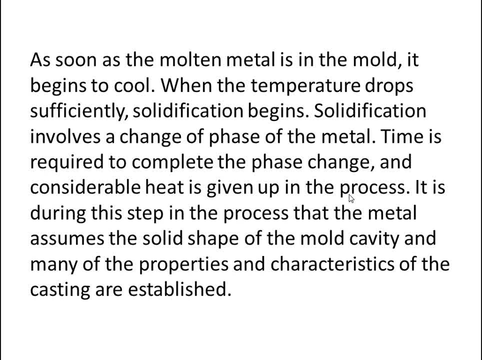 to complete phase change, and considerable heat is given up in the process. It is during this step in the process that the metal assumes the solid shape of the mold cavity and the mold is completely casted. The mold is then casted. Many of the properties and characteristics of the casting are established. 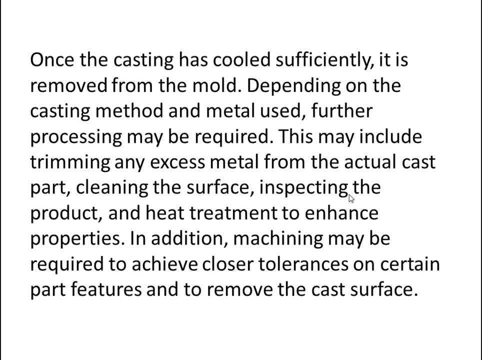 Once the casting has cooled sufficiently, it is removed from the mold. depending on the casting method and metal used, Further processing may be required. This may include trimming any excess metal from the actual cast part, cleaning the surface, inspecting the product and heat treatment to enhance properties.